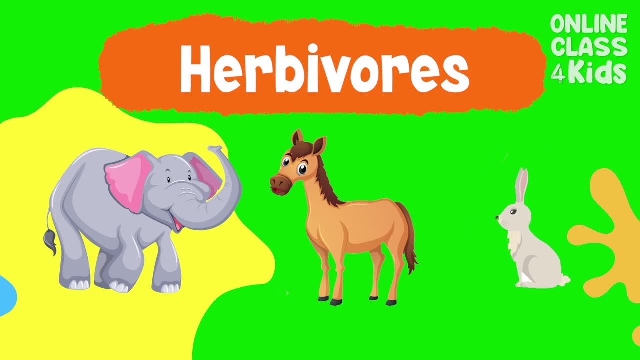 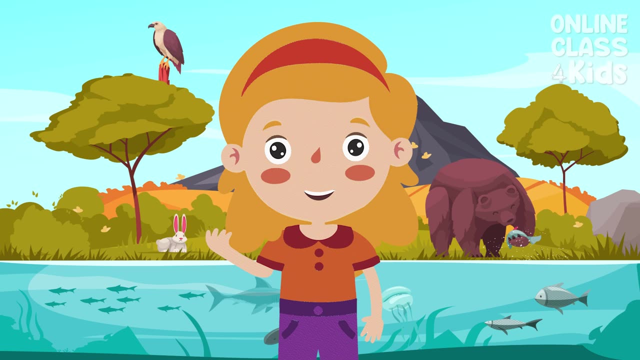 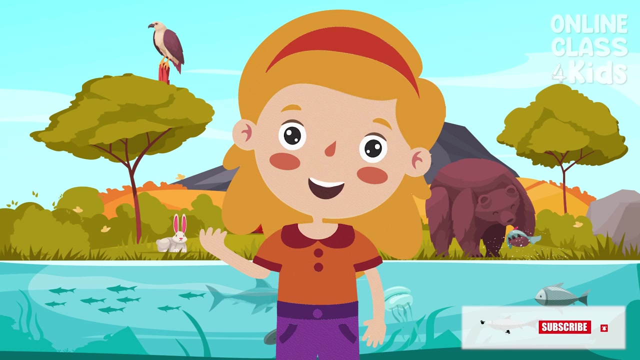 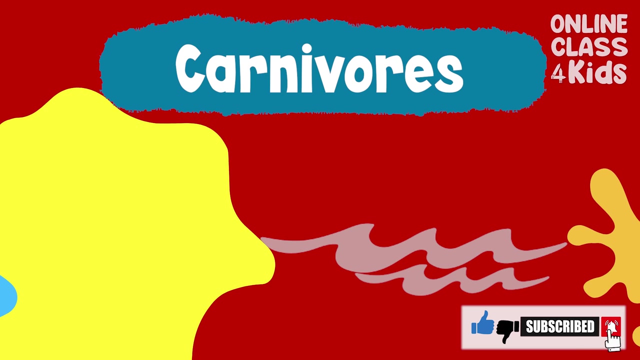 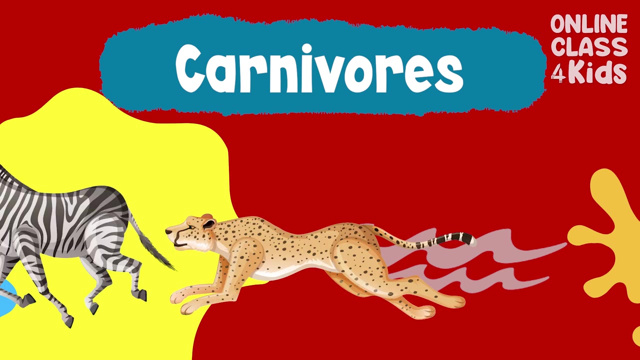 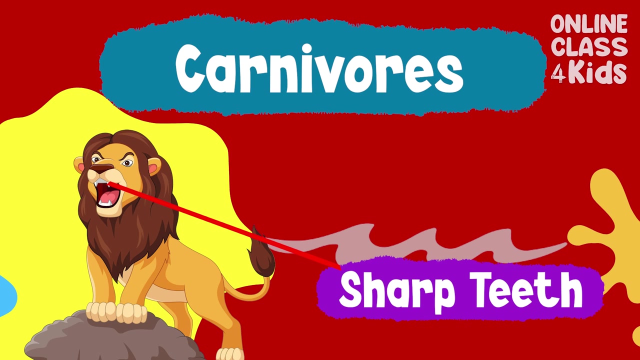 examples of herbivores are elephant, horse and rabbit. can you think of any other animals that only eat plants? great, you are such a smart kid. the second group are the carnivores. these are the animals that only eat meat. they hunt down their prey and they also have stronger jaws and sharp teeth to help them tear up the meat. 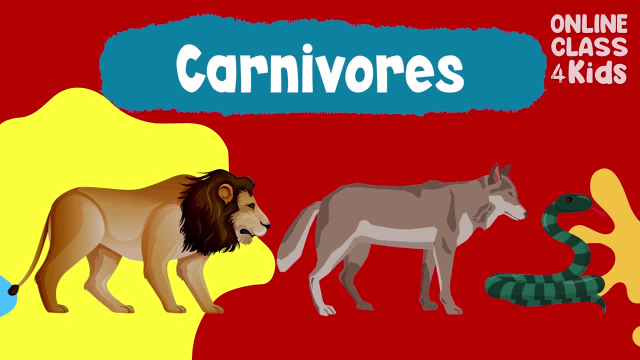 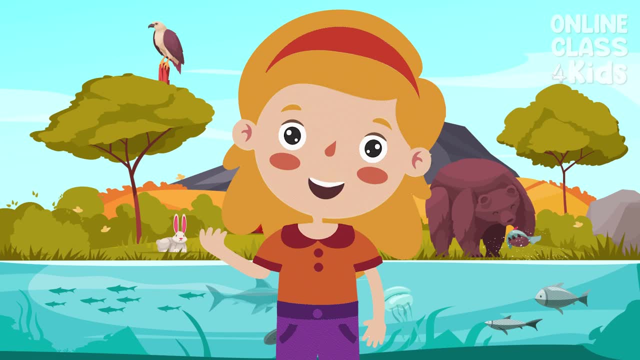 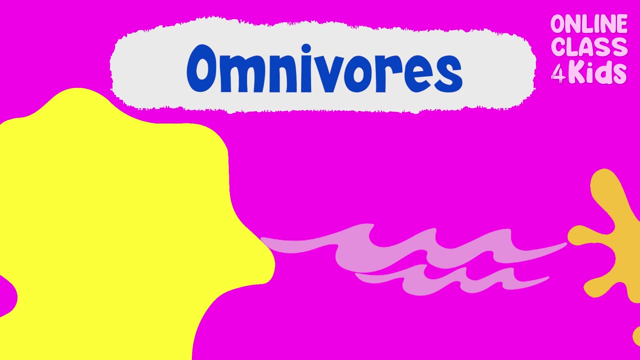 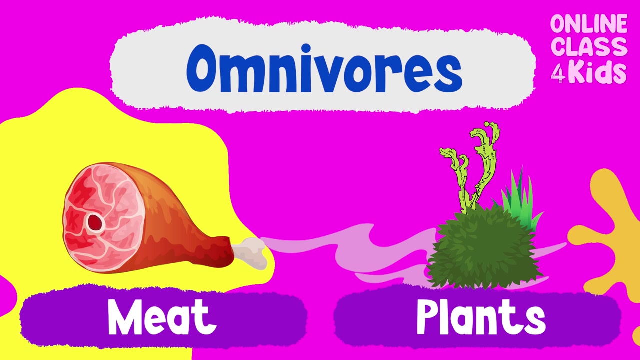 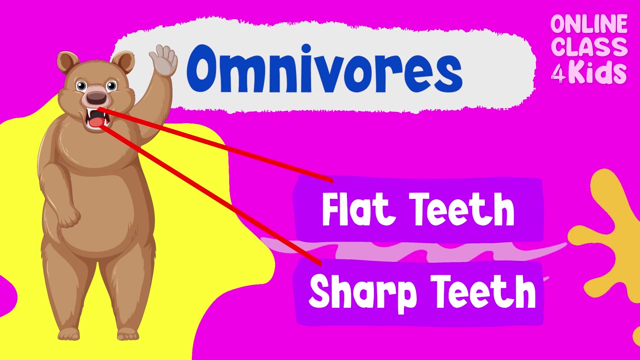 lion, wolf, snake are some of the examples of carnivores. do you know what other animals belong to this category? awesome, you're right, and omnivores are animals that eat both meat and plants, depending on what is abundant or available. omnivores have a combination of flat and sharp teeth, as they eat both kinds of food. 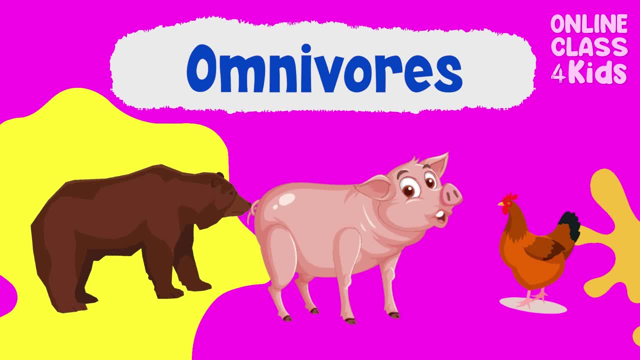 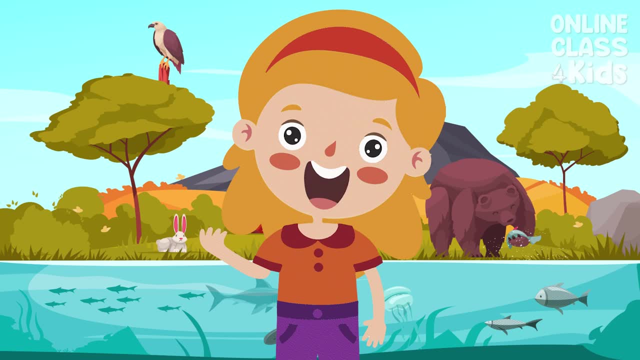 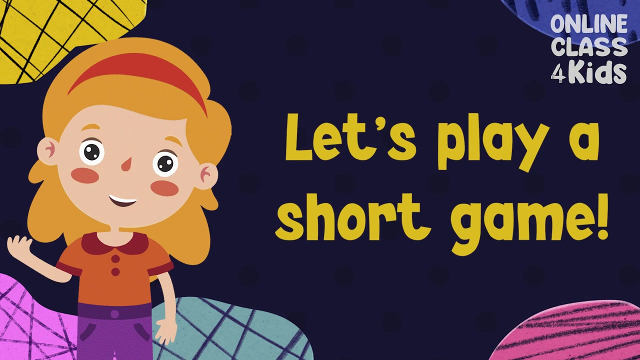 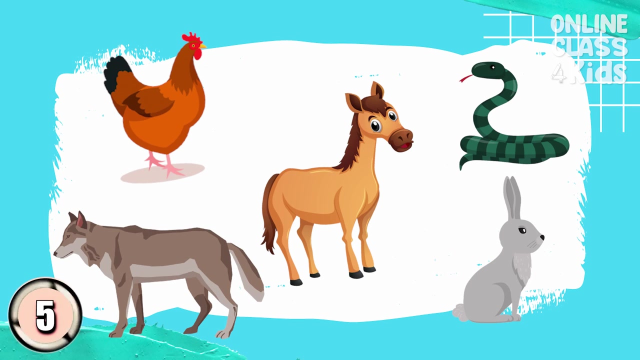 bear, cake and chicken are examples of omnivores. can you name any other animals that are omnivores? very good, now let's play a short game. choose the animals that are herbivores. choose the animals that are herbivores. choose the animals that are herbivores. 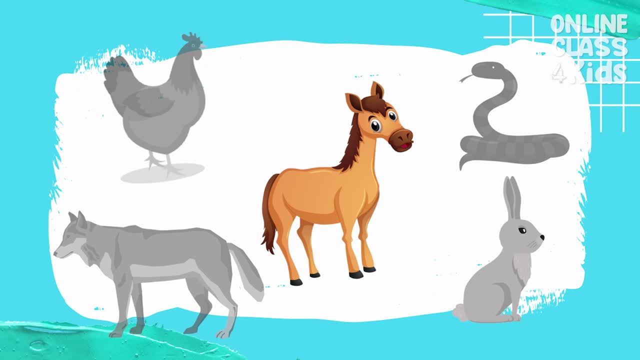 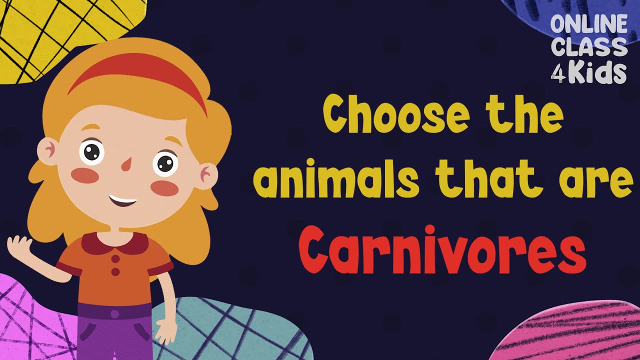 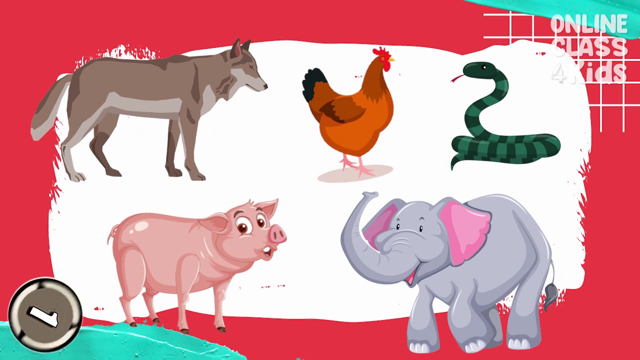 if you play on the stage with your dorm. Sichuan, those deals are expensive. andimming USB, habrido. yes, let's play on the stage with alguém else? excellent, the answers are snake and wolf. if you play on the stage with your dorm, you can getLook at four animals. every other animal is carnivor. Well, that's it. now let's learn to play with snakes. it's pretty easy to play with snakes lives if you are in your first tenants or simply residing in a community. we will teach you how to use all animals them. that're flavor herbivores and insect bomes- excellent, but the answers are snake and wolf. you will see the animals that you leven, andוש ZackHHH, The answer is a snake and wolf and the animals that are carnivores. if you live in the city and live in our place, choose the animals that are carnivores, okay, Drive so you can buy the animals and keep their lives.